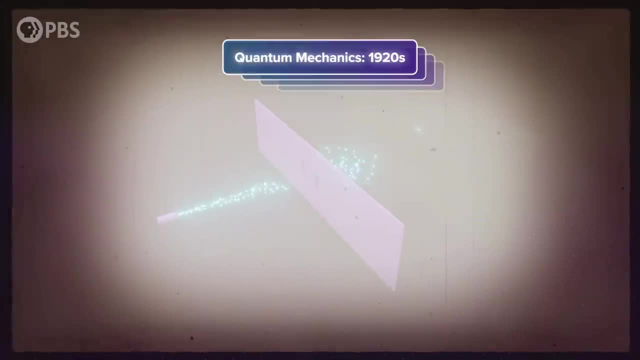 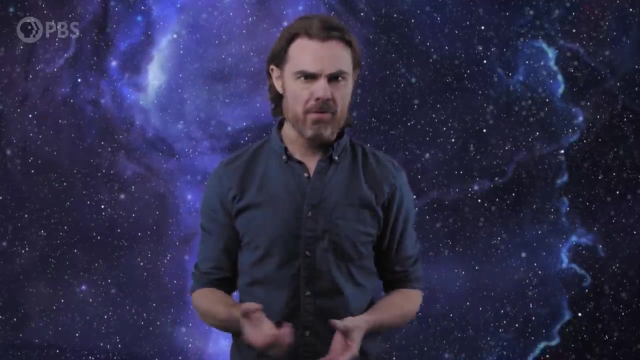 we discovered quantum mechanics, which would become our modern theory of everything except gravity. It was an exciting decade or so for physics, but then things slowed down. We've spent the following hundred years trying to reconcile these two theories and bring them together into a single master theory of everything, The most common approach to this reconciliation. 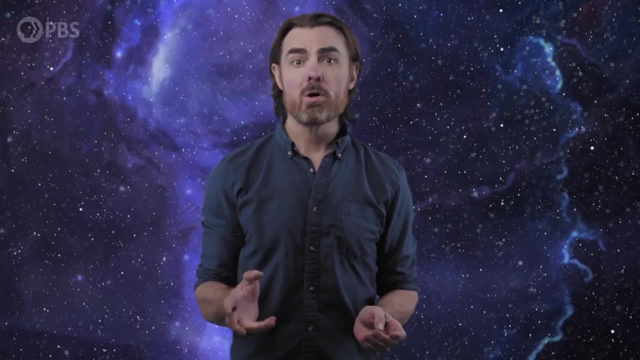 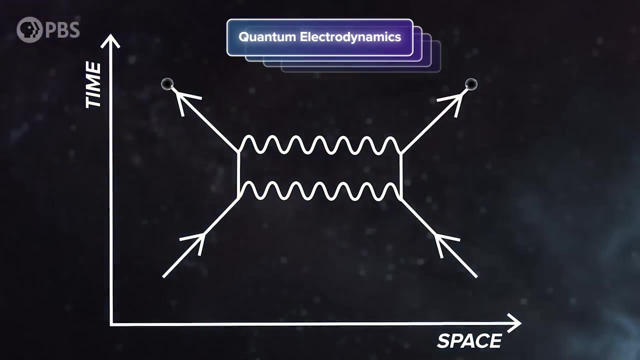 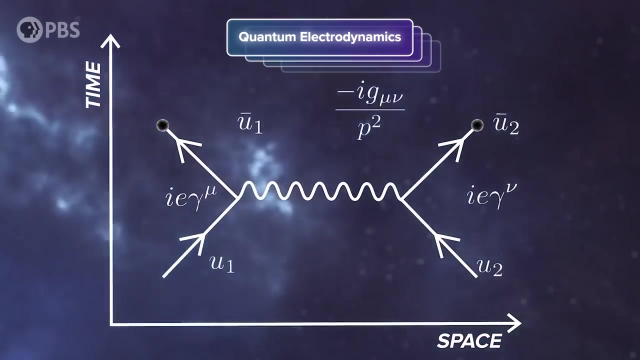 has been to try to make gravity quantum. After all, we got a theory of quantum electromagnetism by quantizing the electromagnetic field. The result was quantum electrodynamics, in which the force of electromagnetism can be described by the exchange of a single quantum of this field, which turns out to be the photon. The same basic procedure. 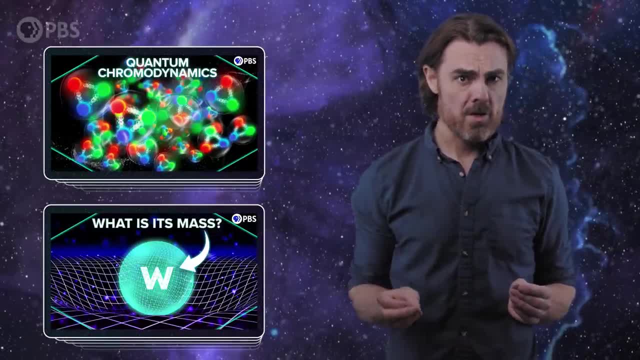 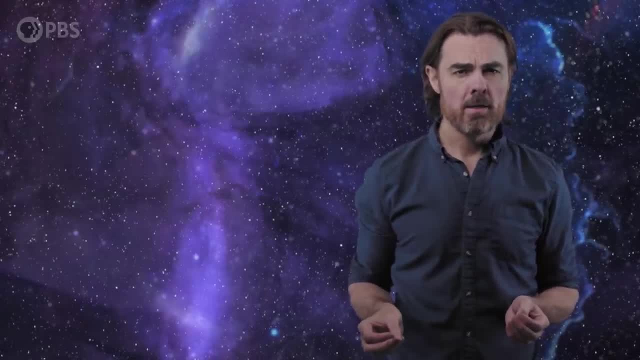 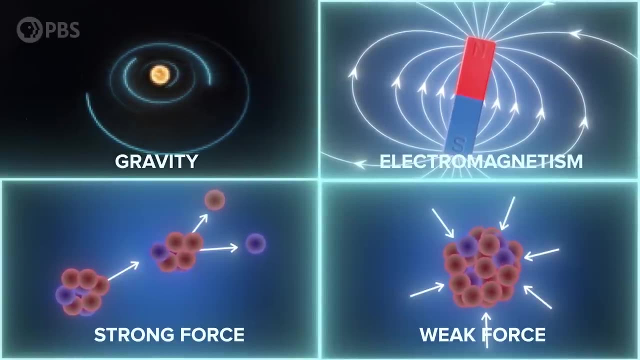 led to the discovery and quantization of the strong and weak nuclear forces, with their association with gravity – And, in practice, love is made of all Cu particles – ambulance molecules, gluons carrying the strong force, and W and Z bosons carrying the weak. 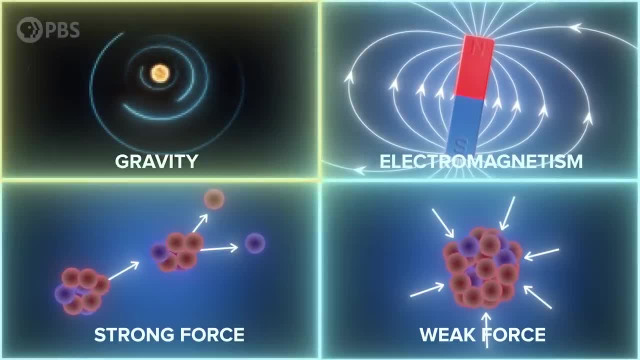 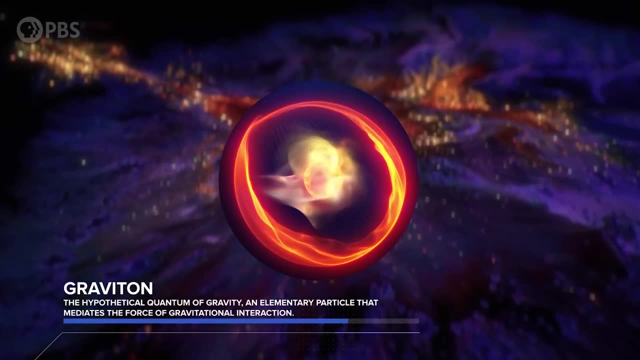 So if three of the four forces of nature are quantum, surely quantizing gravity is an essential step on the path to a final theory? And if the gravitational field is quantized, then it should be made up of quanta – gravity should be mediated by its own force carrying. 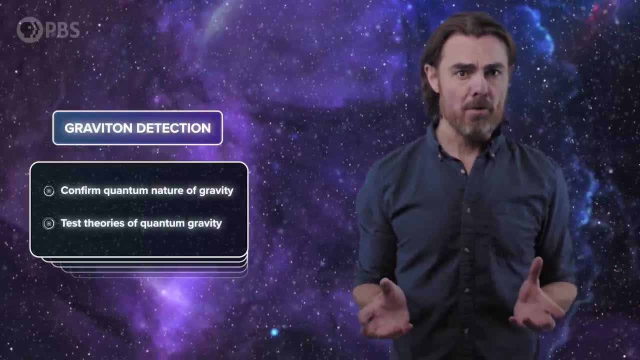 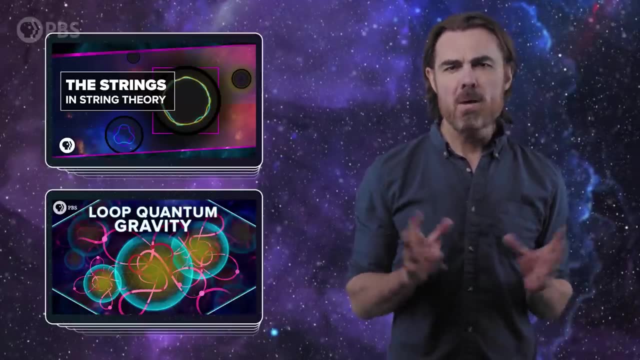 firm gravity's quantum nature and even test our theories of quantum gravity, such as string theory and loop quantum gravity. We've talked about these theories in the past. They are mathematically very dense and involve quite a bit of speculation, and some have. 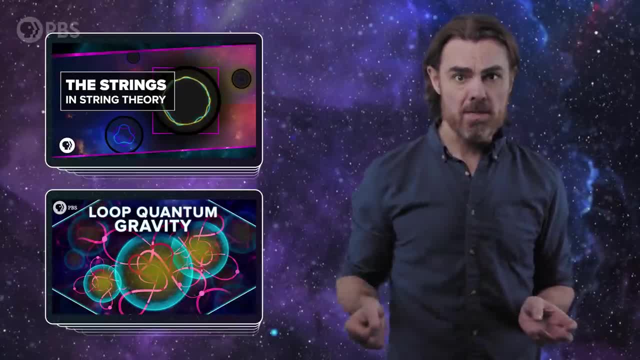 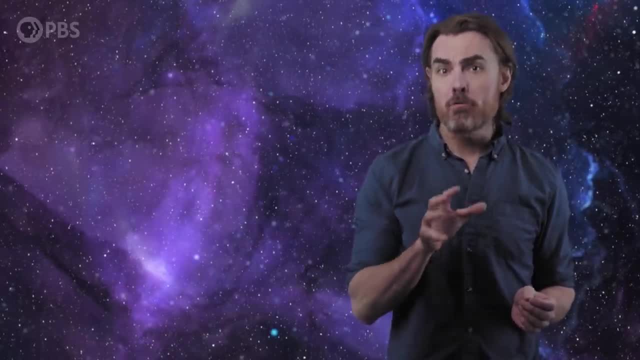 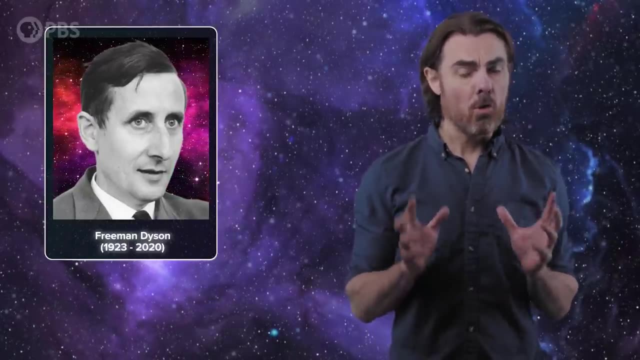 argued that we are getting way, way ahead of ourselves with these theories. So today we're going to get right back to the basics. To do that, we'll follow some of the thinking of Freeman Dyson, who helped shape quantum theory from near the beginning and thought about the most fundamental questions for all. 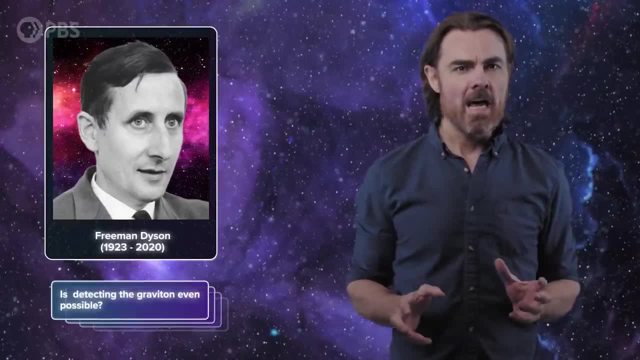 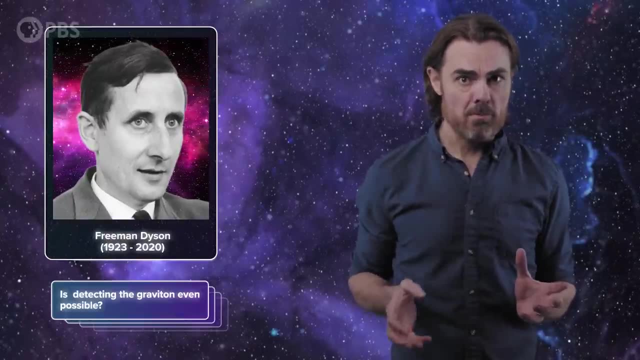 his long life. We'll see what he had to say about whether it's even possible to detect a graviton, something we need to do in order to verify that gravity really is quantum. But first we're going to follow another musing of Dyson's, in which he asks whether 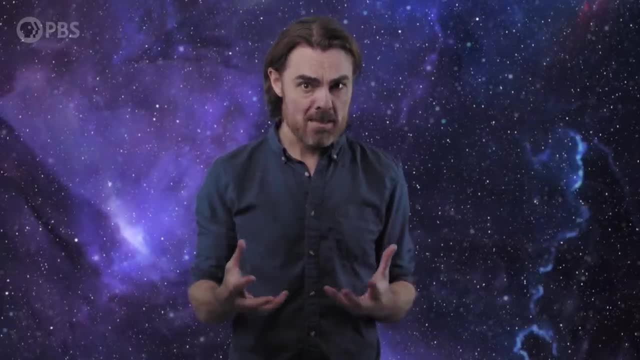 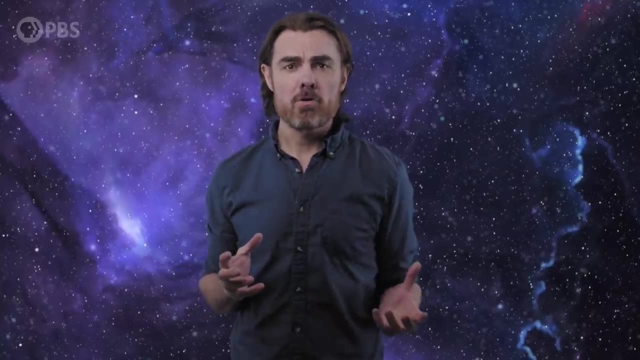 the same trick that told us that electromagnetism must be a quantum force can also be applied to gravity. The quantum nature of electromagnetism is the same as the quantum nature of quantum energy. It was the very first clue that led to the quantum revolution. 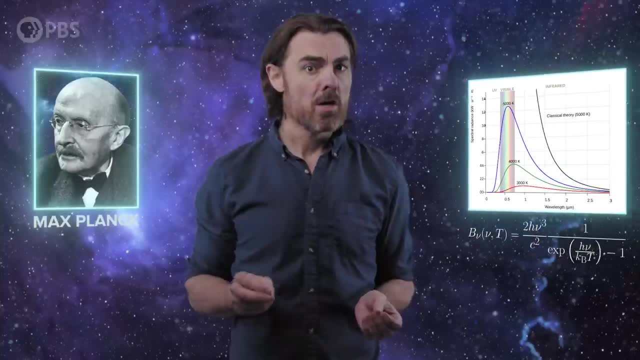 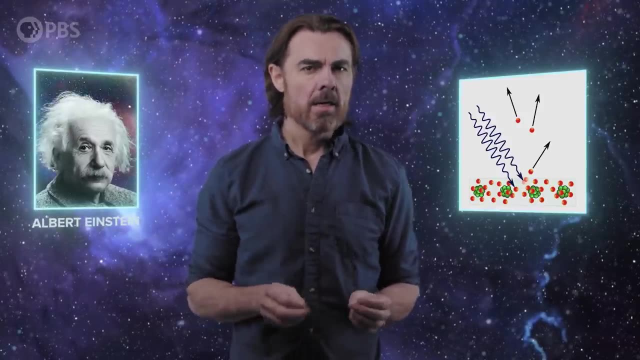 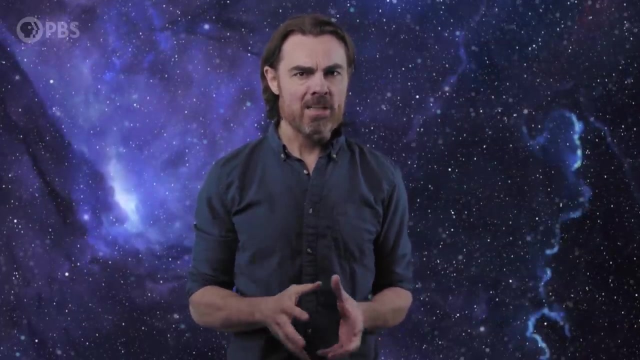 It first showed up in the mathematical trick that Max Planck used to explain thermal radiation, and this inspired Einstein to take the quantization of electromagnetism seriously in order to explain the photoelectric effect. Now we understand that the electromagnetic field and electromagnetic waves, aka light, 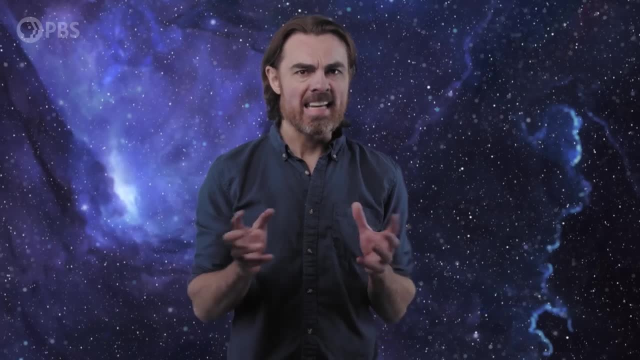 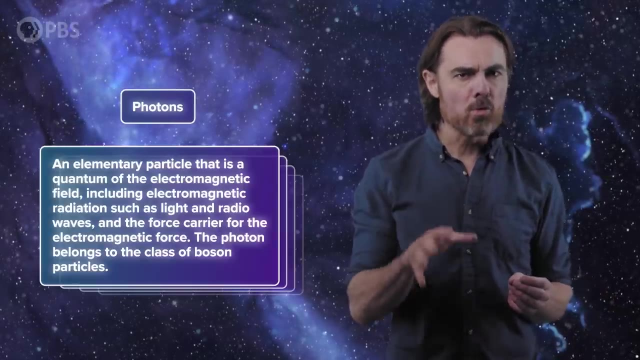 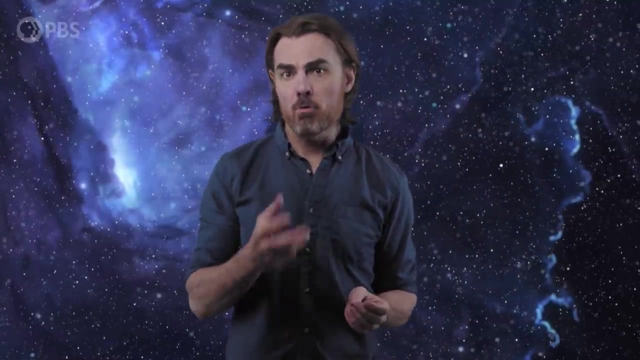 can be described as being composed of countless tiny and individual packets of energy called photons. Planck and Einstein's discoveries were clues that led to the full development of quantum mechanics in the mid-1920s, which was followed quickly by our full quantum theory of electromagnetism. 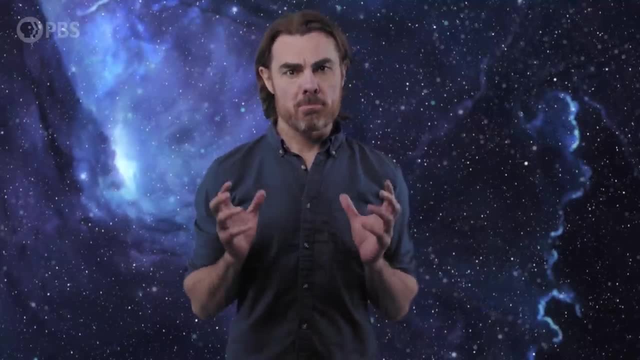 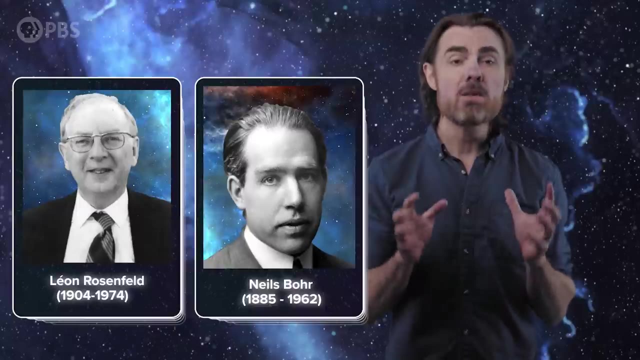 quantum electrodynamics. But even before electromagnetism was properly quantized, Niels Bohr and Leon Rosenfeld came up with a strong argument that this force must be fundamentally quantum. I'm going to go through this thought experiment. I'm going to go through this thought experiment. 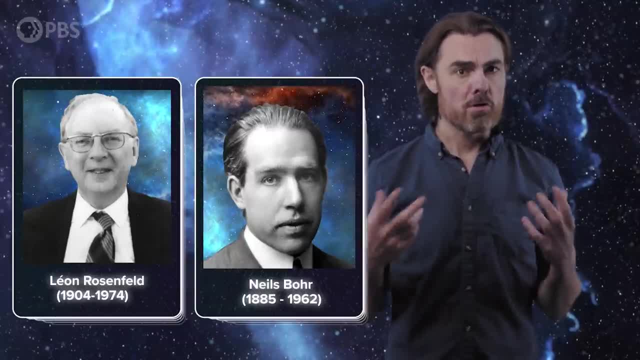 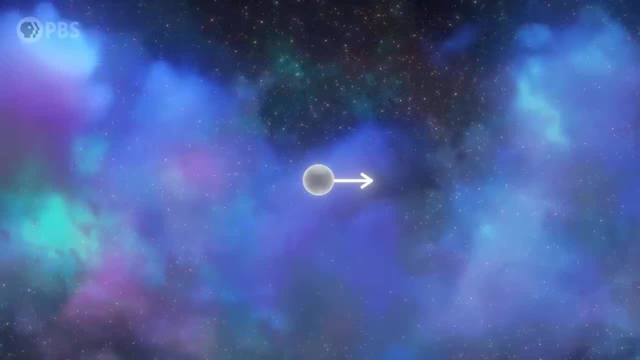 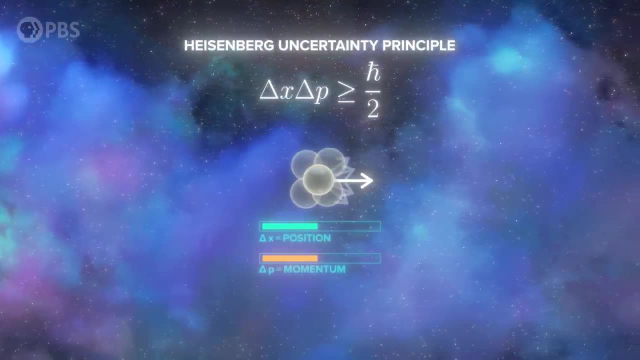 Because maybe if it works for electromagnetism, we can also use it to argue for gravity being quantum. Let's start with a simple particle in motion. At any point in time, a particle has a position and a momentum. If this is a quantum particle, then it is impossible to simultaneously measure both. 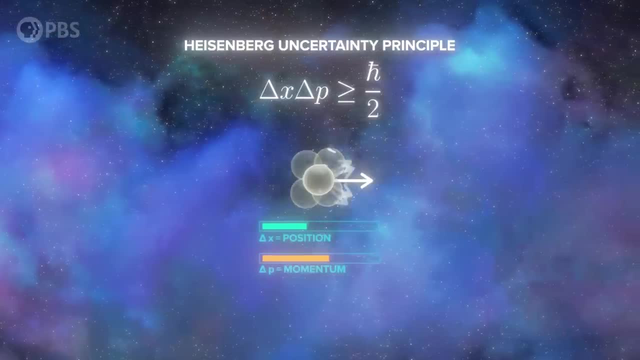 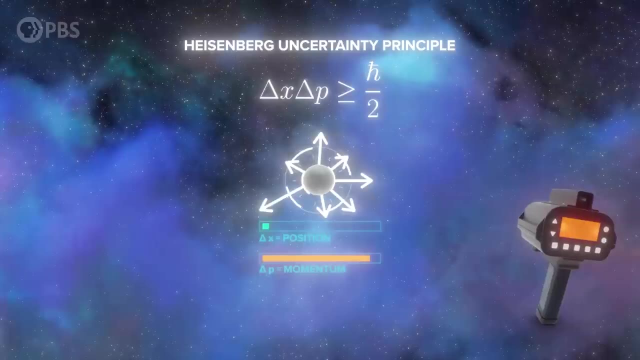 of these properties with perfect precision. If we try to measure the position very precisely, then the uncertainty in the momentum increases. If we try to measure the momentum as perfectly as possible, then the uncertainty in the momentum increases. If we try to measure the momentum as perfectly as possible, then the position becomes undefined. 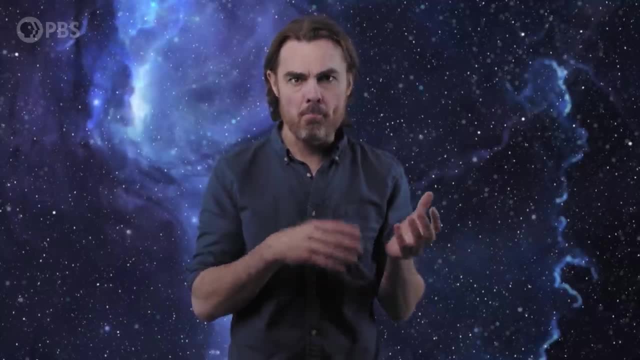 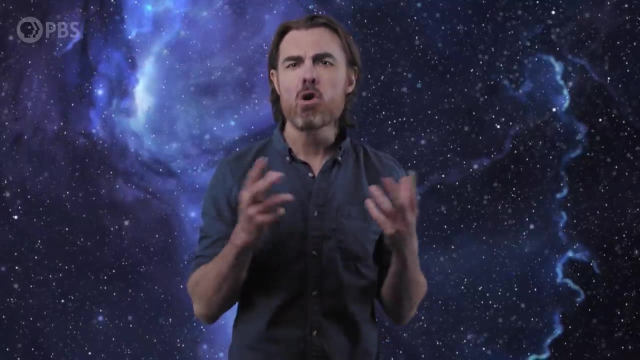 And it's not just that we lost the certainty in one property by bumping it or whatever, when we tried to measure the other. The Heisenberg uncertainty principle is a fundamental limit to the knowability of the quantum world, and we talk about this fundamentalness in this video. 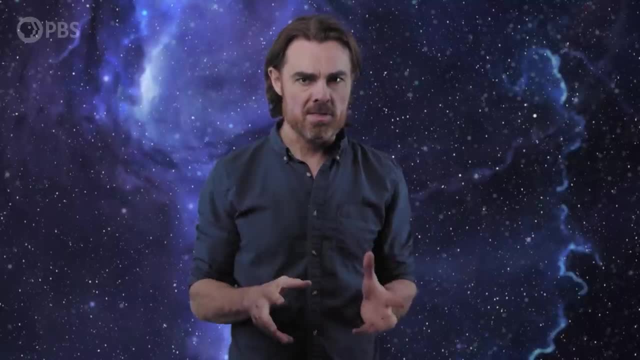 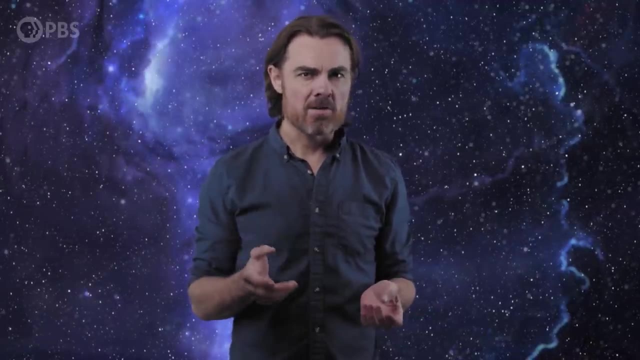 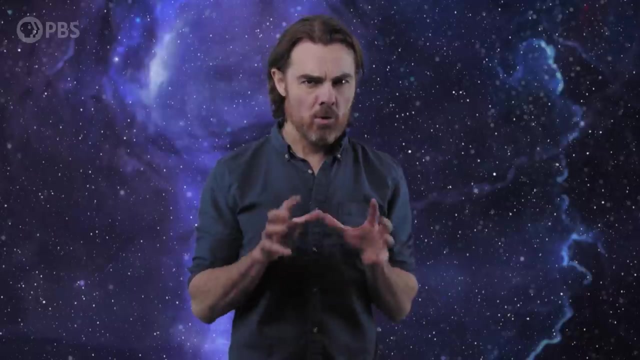 This trade-off between the knowledge we can possess about a quantum system applies to many pairs of properties: Position versus momentum, Energy versus time, One axis of polarization or spin versus a perpendicular axis, and many more. So, if the electromagnetic field is quantum in nature, the uncertainty principle should 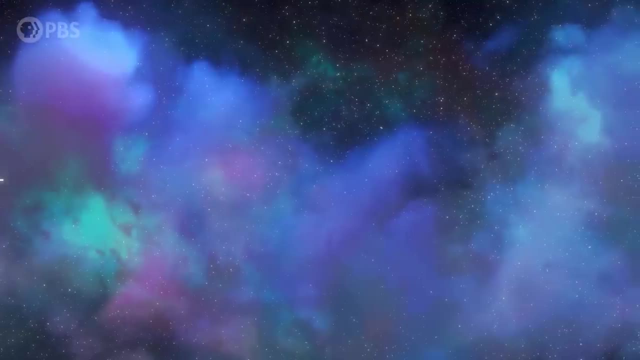 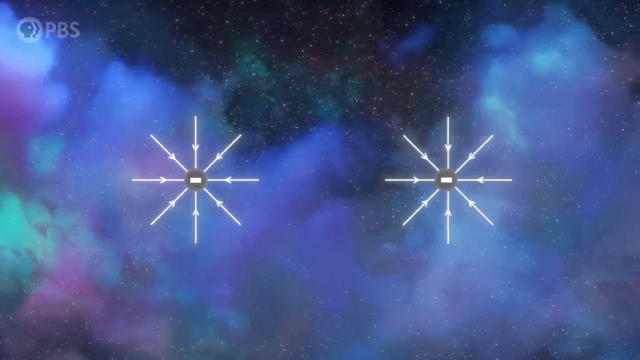 apply to our attempts to measure this field. Okay, back to our particle. In fact, let's have two particles and give them both a negative electric charge. We start them off moving towards each other. We know that light charges repel, so these particles will interact by the electromagnetic. 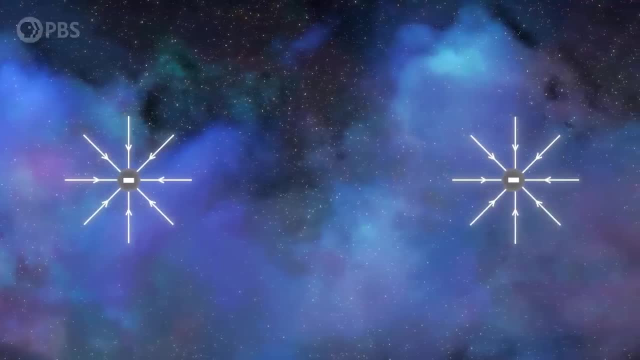 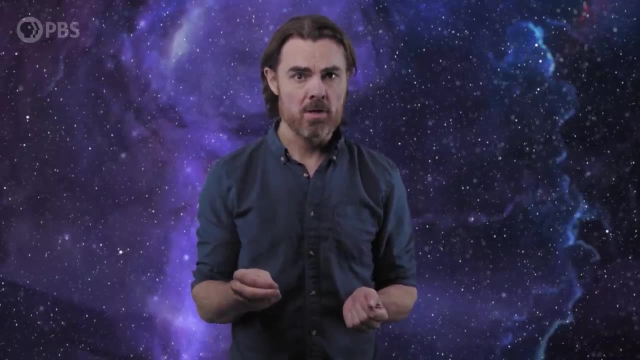 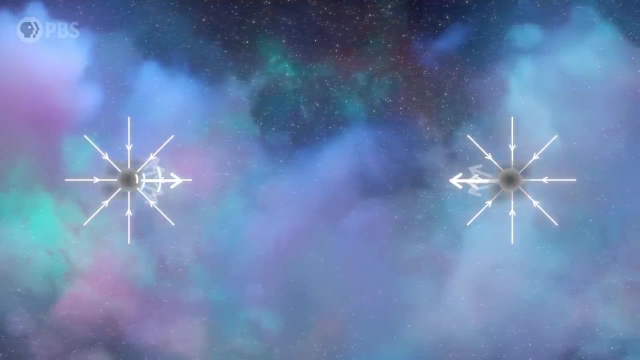 field when they get close and be deflected back. We know that there's a quantum restriction on how precisely we can measure the position and momentum of these particles, but we also know that the particles' motions are entirely defined by their interactions via the electromagnetic field. 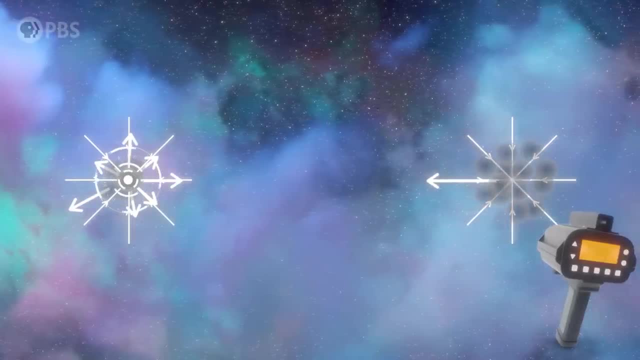 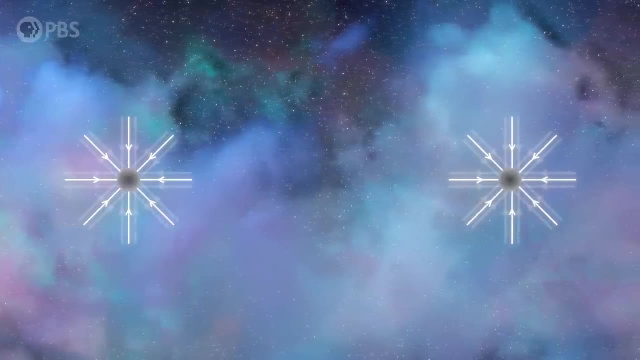 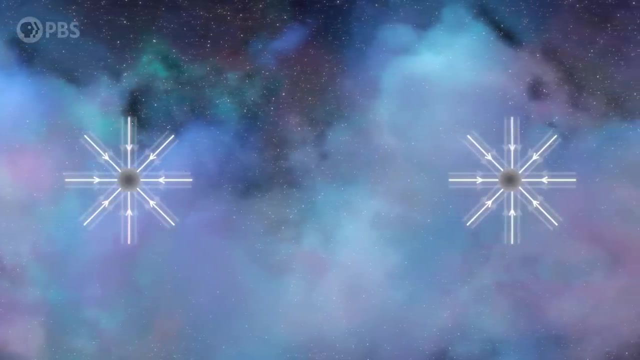 So Bohr and Rosenfeld argued that the same restrictions on measurement of particle motion have to apply to the field that governs that motion. After all, measurements of the electromagnetic field can only happen by observing its interactions. so if these interactions are subject to fundamental quantum uncertainty, then the field must. 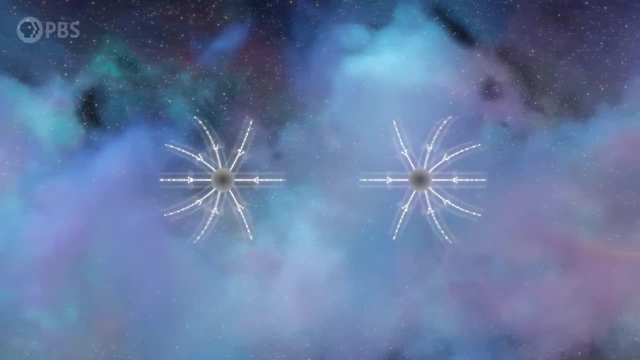 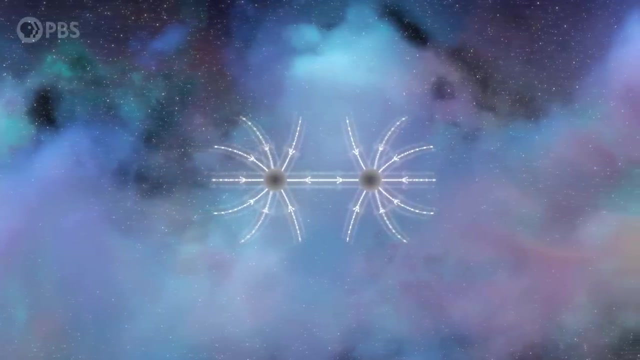 be also, And if that's true, then it's reasonable to think that the electromagnetic field is truly a quantum entity, as indeed it turns out to be Okay. so if this argument applies to electromagnetism, why can't it also apply to the gravitational? 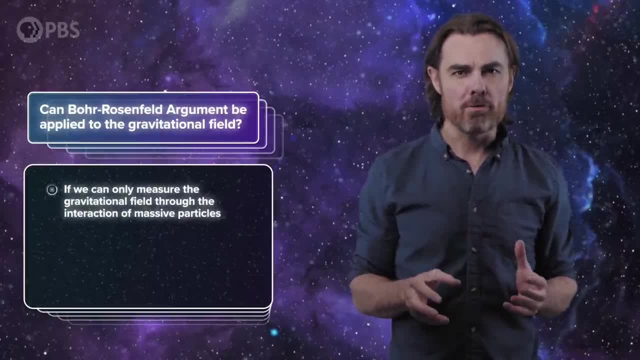 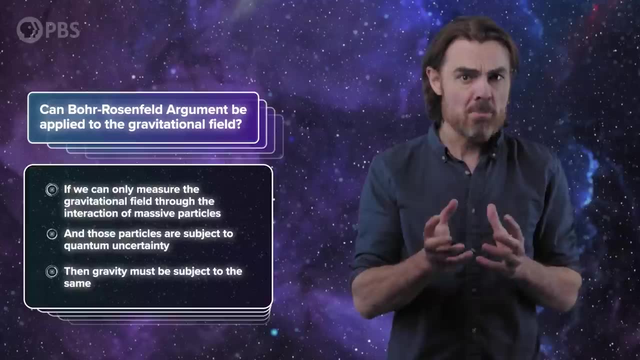 field. If we could only measure the gravitational field through the interaction of massive particles and to quantum uncertainty, then surely our measurement of gravity is subject to the same. Here it's important to pay attention to the details of the Bohr-Rosenfeld argument. 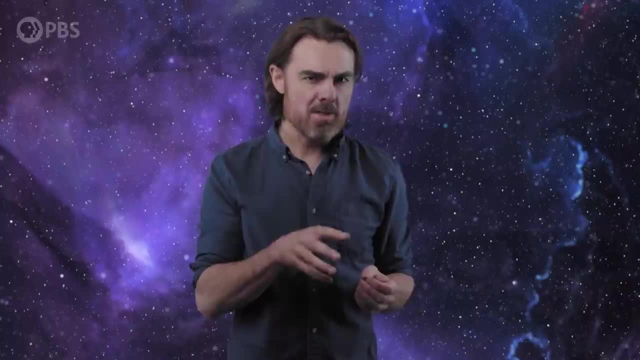 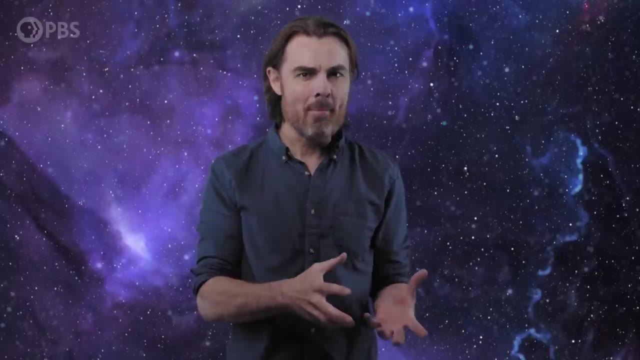 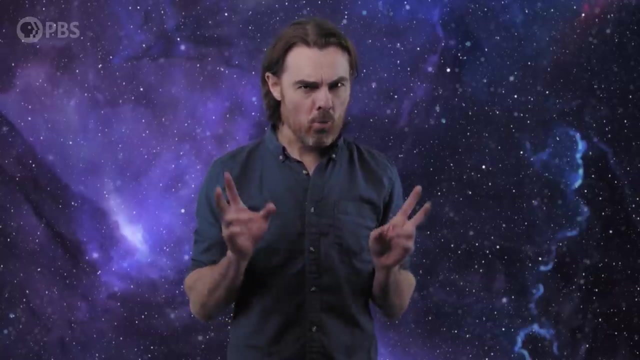 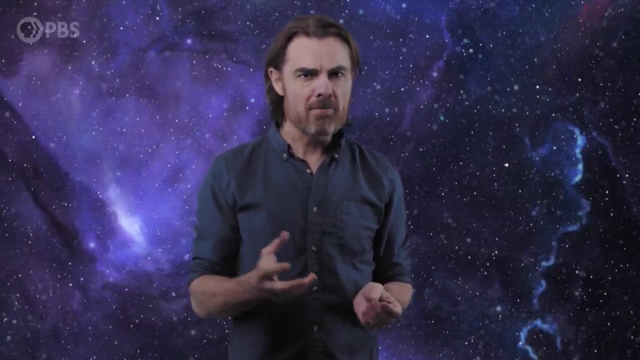 They realized that in order to confidently state that the Heisenberg uncertainty principle applies to electromagnetism, we need to consider only a pristine electromagnetic interaction between the two particles. The interaction needs to be mediated by the most quantum-possible influence of the EM field, a so-called quantum of action. That's the part of the EM field. 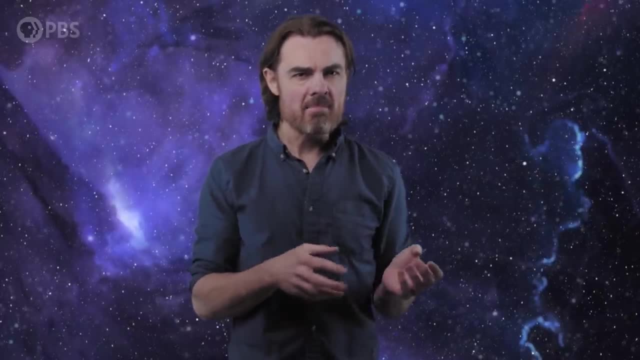 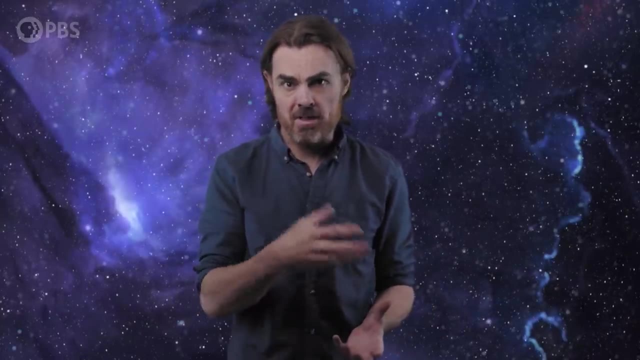 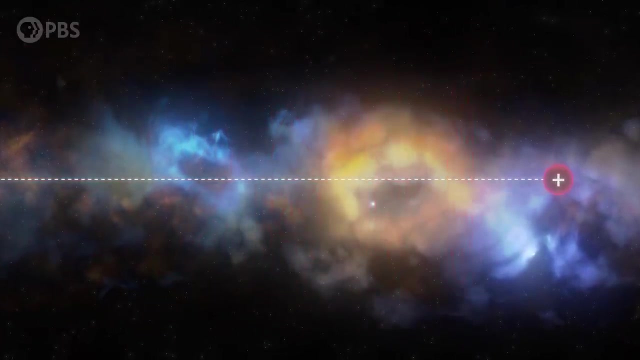 that we're trying to measure. If there are any extra bits of electromagnetic field, then they'll add to our uncertainty in measuring the field responsible for the interaction. But electromagnetism is pretty messy. For example, we know that moving charges create magnetic fields. Those extraneous components of the EM field prevent us from concluding. 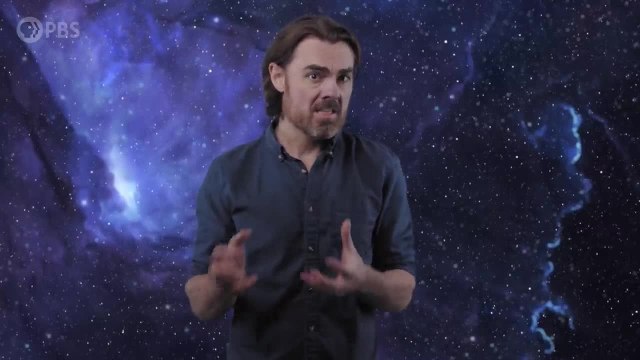 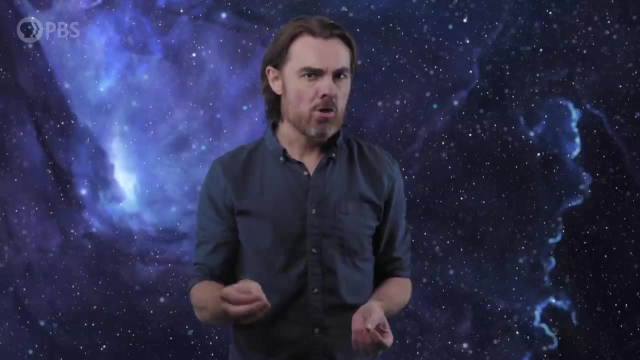 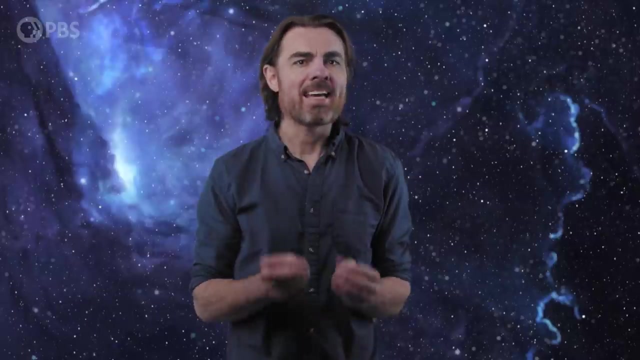 that our knowledge of the EM field is limited to the same degree as our knowledge of particle motion. Only with a pristine interaction can we show that electromagnetism also obeys the Heisenberg uncertainty principle. But Bohr and Rosenfeld came up with a clever trick to clean up the EM. 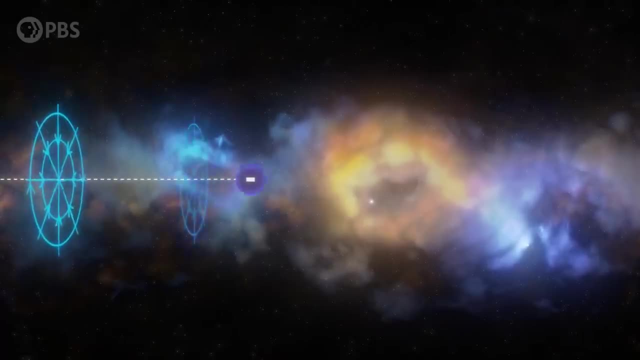 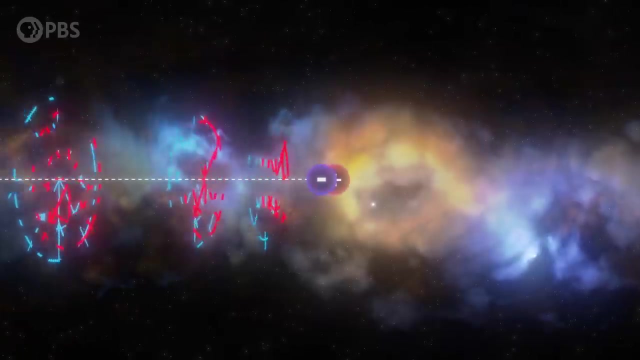 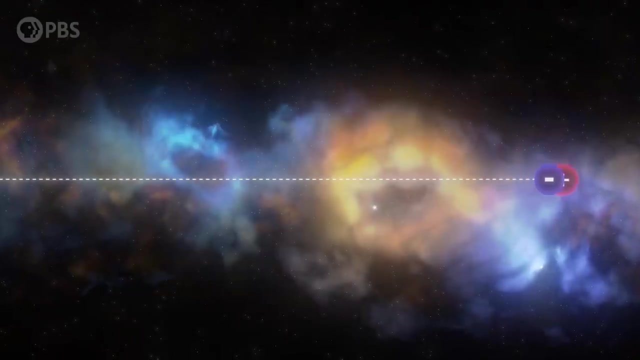 field. in their thought experiment, Instead of individual particles moving towards each other, they imagined inter-particles, one positive and one negative. That cancels out any electromagnetic field emerging from the particle motion, allowing us to describe the most fundamentally quantum interaction via the EM field, And it allows 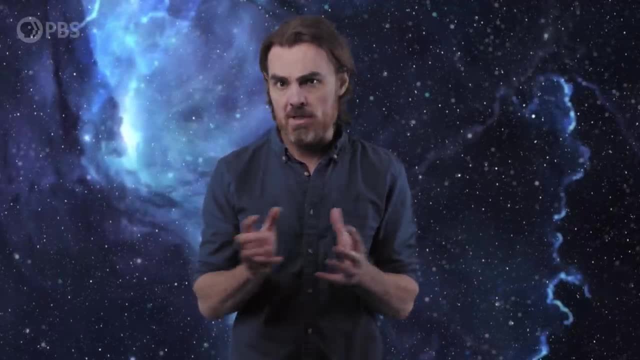 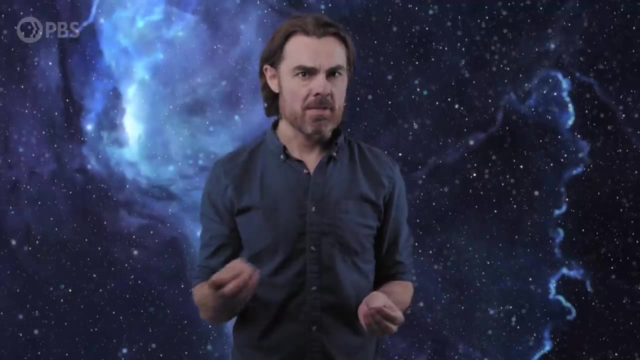 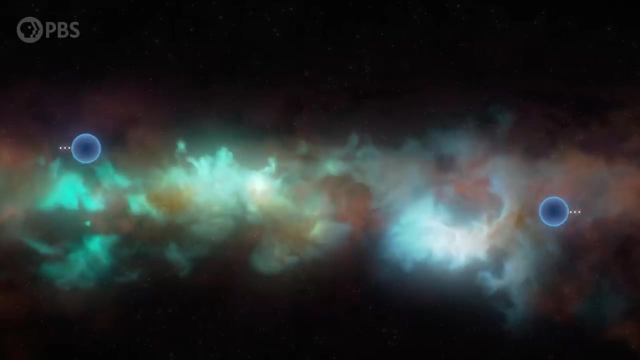 us to show that the EM field really is subject to true quantum uncertainty. But this is where we get stuck with gravity. Particles with electric charge are subject to the electromagnetic force. The analogous charge for gravity is mass. We can imagine a pair of massive particles moving towards each other and interacting via a quantum of gravity. 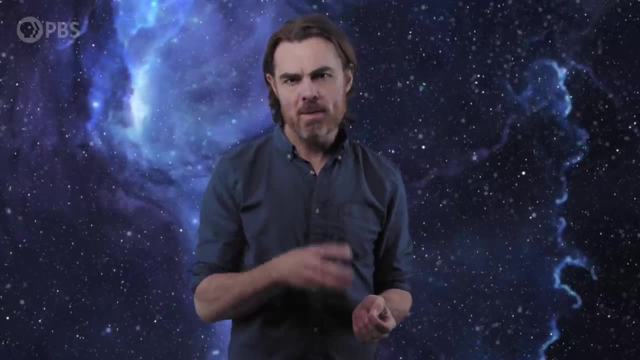 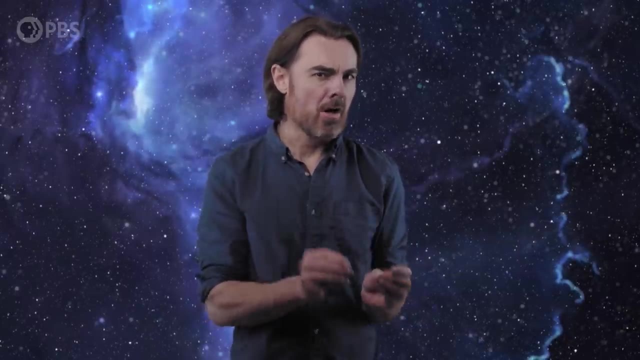 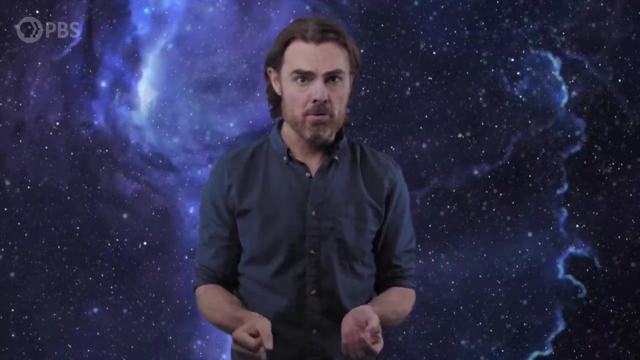 Our ability to measure that gravitational interaction should be limited by our ability to measure the motion of those particles. But in order to show that the limit is truly the Heisenberg limit, we need to rule out complex interactions for the gravitational field, just as we did for the EM field. So why not apply the same trick as Bohr and Rosenfeld? 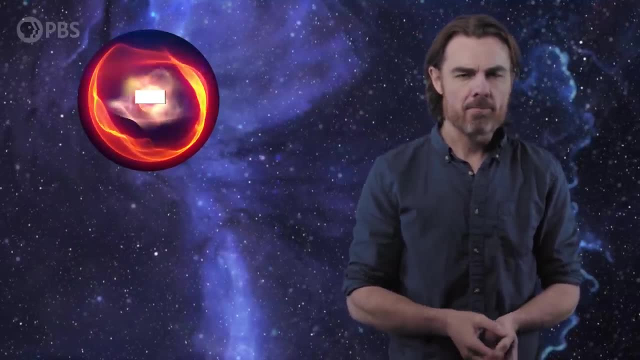 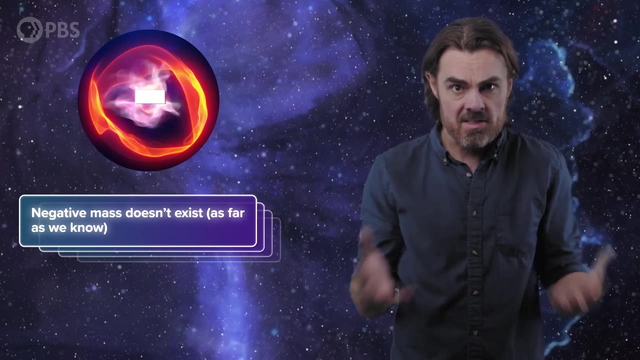 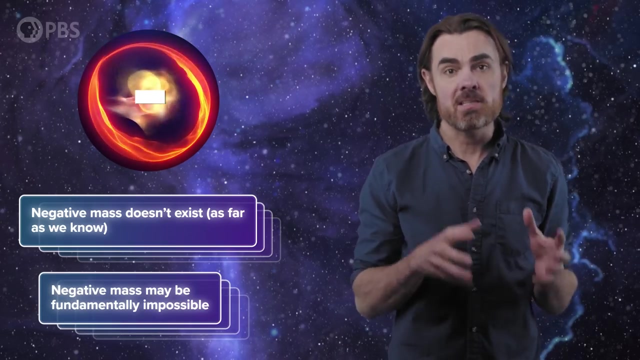 just add an opposite gravitational charge to each particle, But that means adding negative masses. And as far as we know, negative mass doesn't exist. And it's not just that we haven't discovered it yet. There are very good reasons to believe that negative mass is fundamentally impossible. Its existence would lead to major paradoxes. 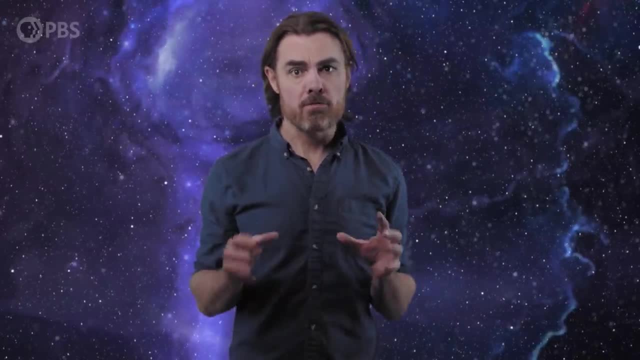 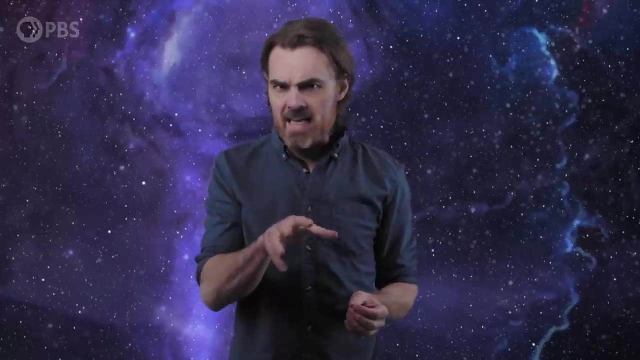 So it seems that the very nature of gravity forbids us from using Bohr and Rosenfeld's argument. That might, on the surface sound like a bit of bad luck, but follow me through the next thought experiment and it starts to feel like the universe is really conspiring to prevent us. 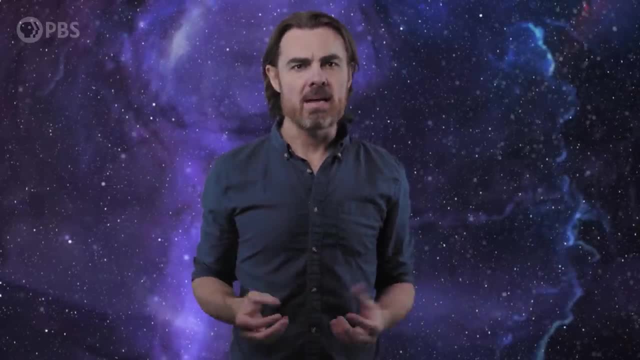 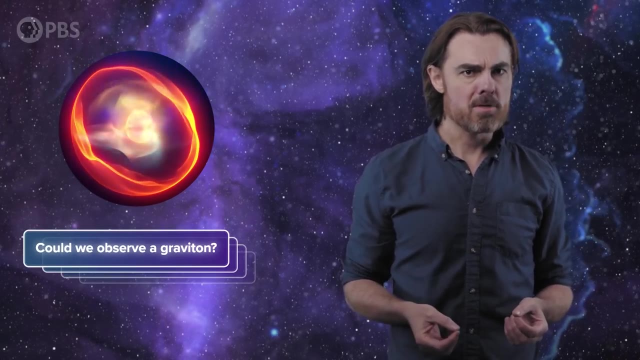 from finding evidence of quantum gravity. Perhaps the most direct evidence of quantum gravity would be the observation of a graviton, or at least of its effect. After all, the observation of the influence of individual photons in the photoelectric effect was a pretty clear 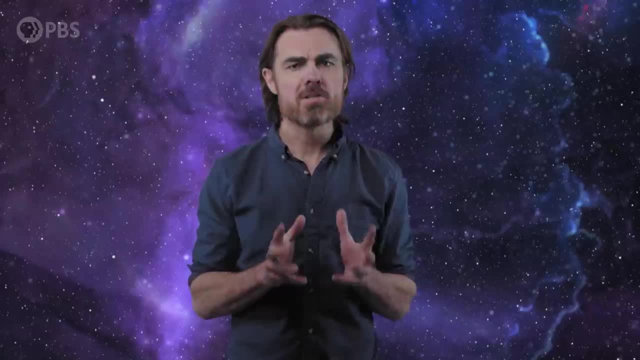 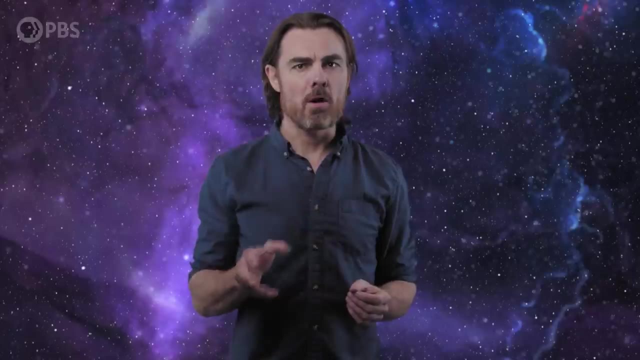 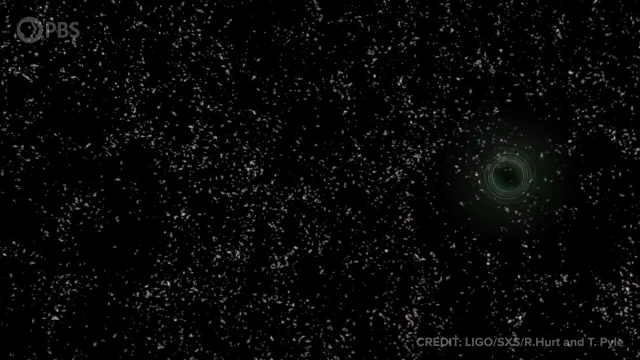 demonstration of the quantization of electromagnetism. So onto the next thought experiment from Freeman Dyson. He figured out what it would take to detect an individual graviton with a gravitational wave detector. Gravitational waves are ripples in the fabric of spacetime caused by massive objects undergoing 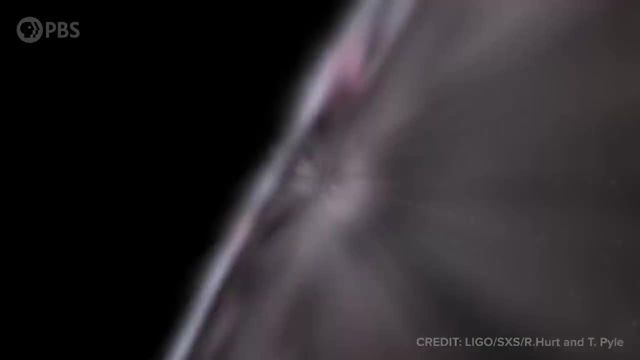 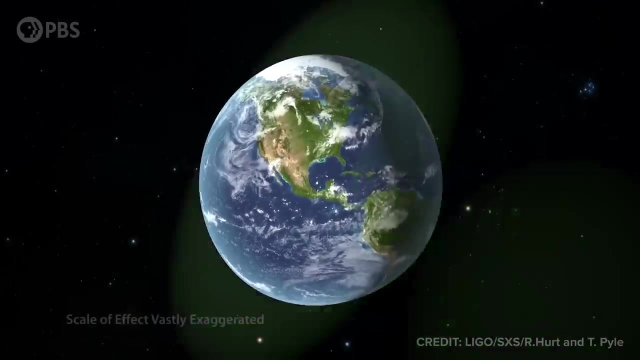 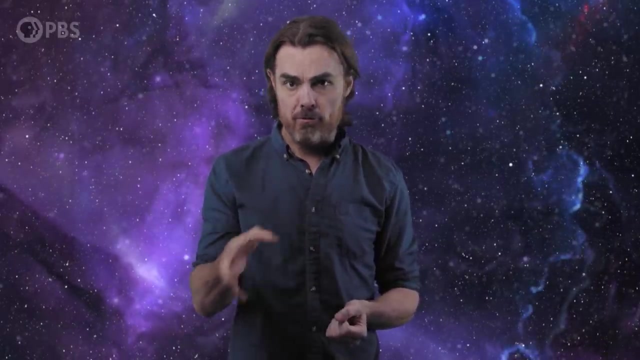 certain types of motion. When a gravitational wave passes by, it causes distances to change, as space is alternately stretched and compacted by a very tiny amount. At least that's how gravitational waves look in general relativity – Einstein's very un-quantum Theory of Gravity. 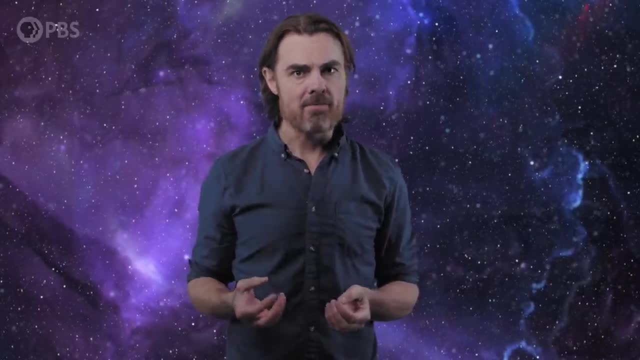 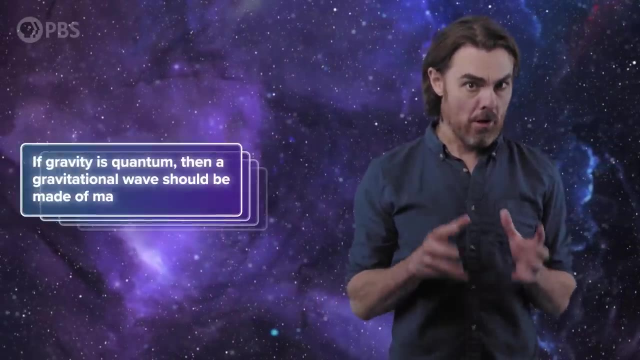 In classical Sovelius' theory of quantum gravity, the gravitational waves are relatively non-quantum electrical electromagnetism. electromagnetic waves are caused by accelerated charges, But we now know that those waves are really made up of individual photons. so if gravity 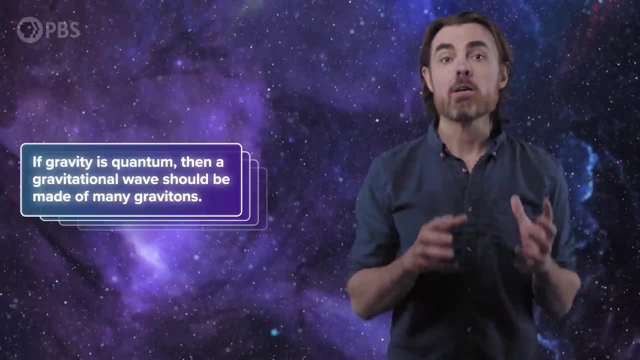 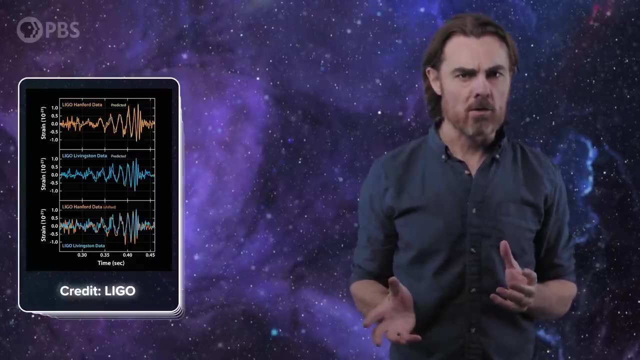 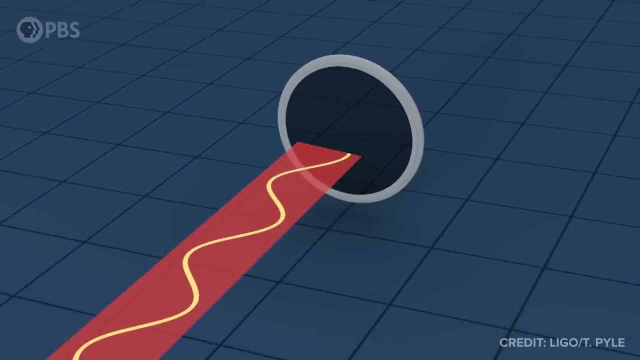 is quantum, then a gravitational wave should be made up of many gravitons. In 2015, we detected our first gravitational waves caused by the merger of black holes. with the Laser Interferometer Gravitational Wave Observatory, The two LIGO facilities sensed the extremely tiny relative changes in the lengths between: 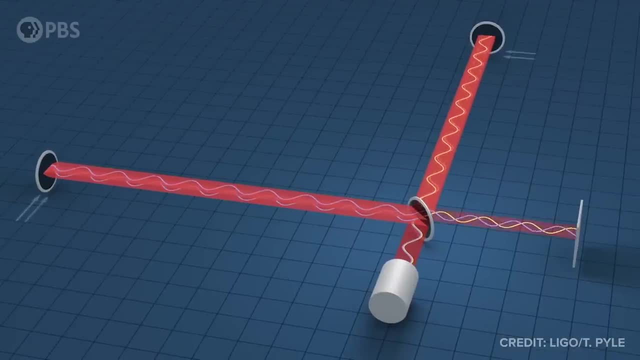 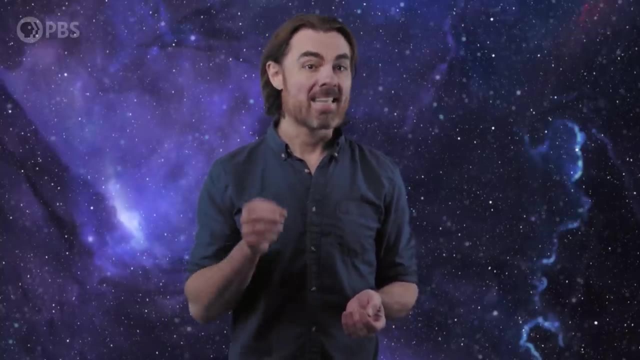 their 4km arms by bouncing lasers many times along each arm and watching for subtle changes in how those beams recombined. So what would it take to measure a single graviton? Probably is quite a bit more difficult than measuring a single photon, but there must. 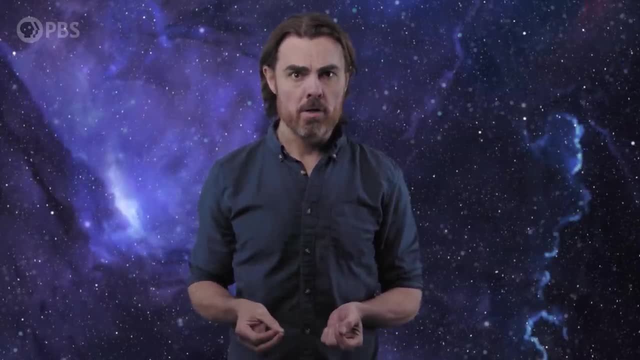 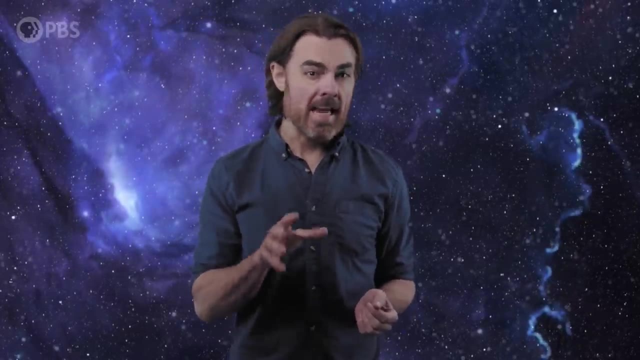 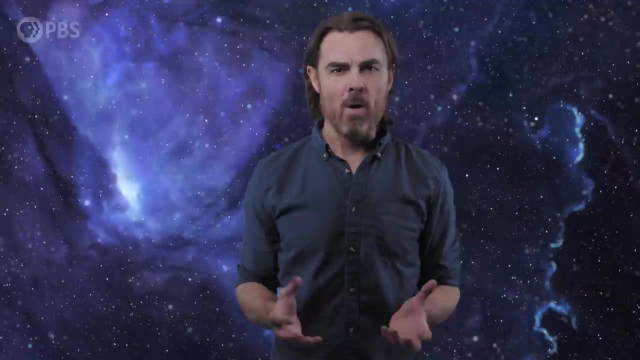 be some far future gravitational wave detector that could do it. That's what Dyson wanted to find out. So we'll start By estimating how many gravitons are in a typical gravitational wave like the ones detected by LIGO. If we wanted to do that for an electromagnetic wave, we take the total energy of the wave. 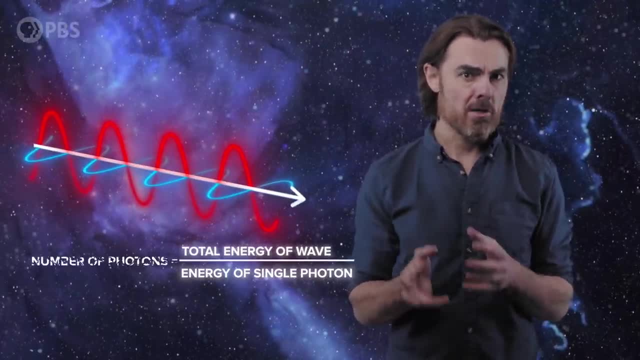 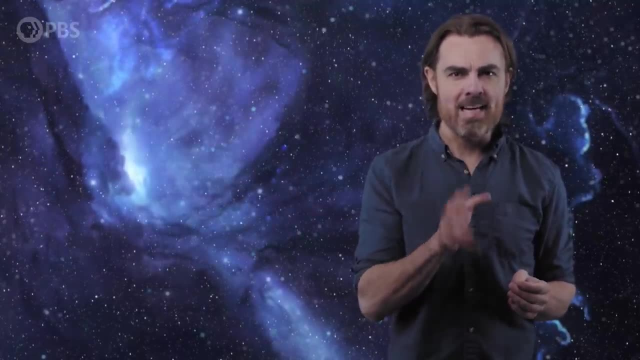 and divide it by the energy of a single photon, which is just the Planck constant times its frequency. That tells us that a piddling 5 milliwatt, 630 nanometer red laser pointer blasts out 10 to the power of 16 photons per second. 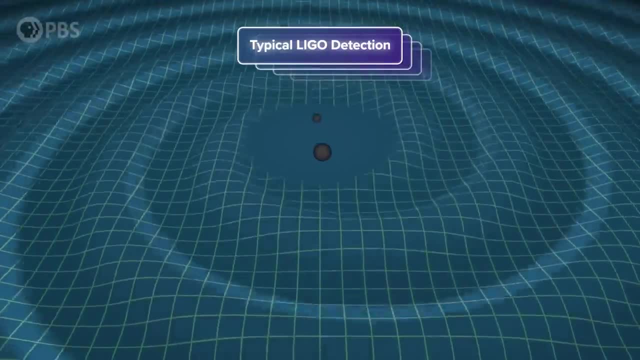 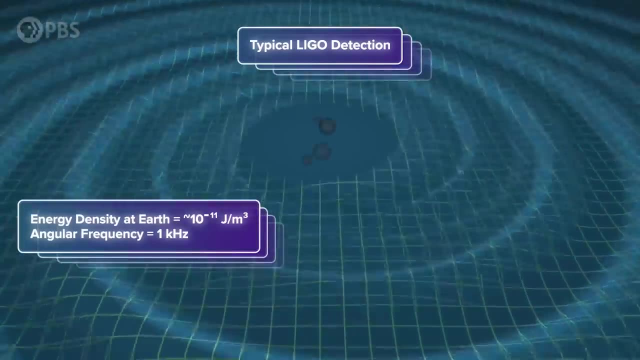 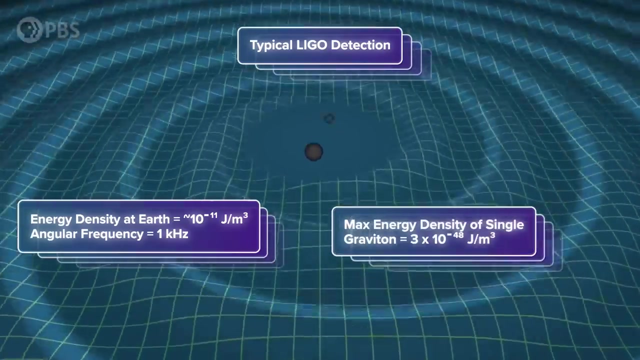 The typical gravitational wave detectable by LIGO has an energy density of approximately 10 to the power of minus 11 joules per cubic meter with an angular frequency of 1 kilohertz, That's a thousand hertz According to Dyson. the energy density of a single graviton in this frequency is at 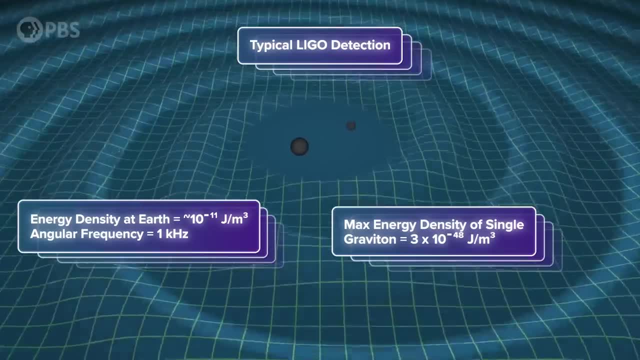 most 3 by 10 to the power of minus 48 joules per cubic meter, and that gives us around 3 by 10 to the power of 37 joules per cubic meter. That's a thousand hertz. That's a thousand hertz. 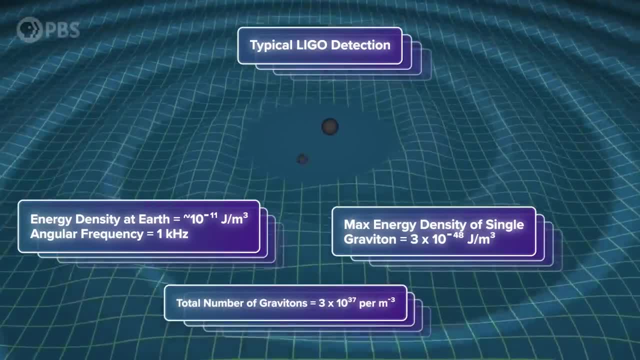 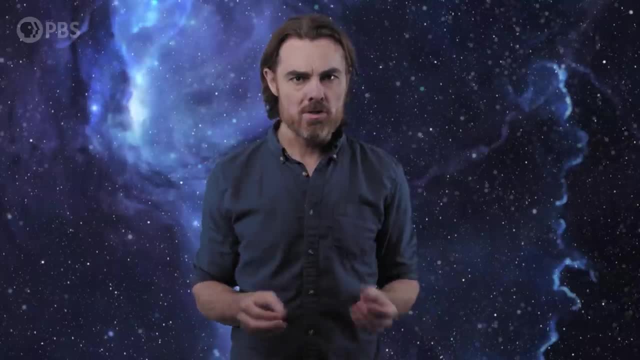 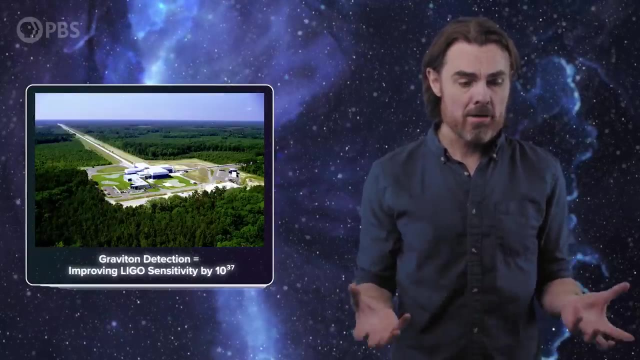 Well, if the gravitational wave that I described has around 10 to the 37 gravitons- and that's just at the edge of LIGO sensitivity- then we need to improve that sensitivity by a factor of 10 to the power of 37.. 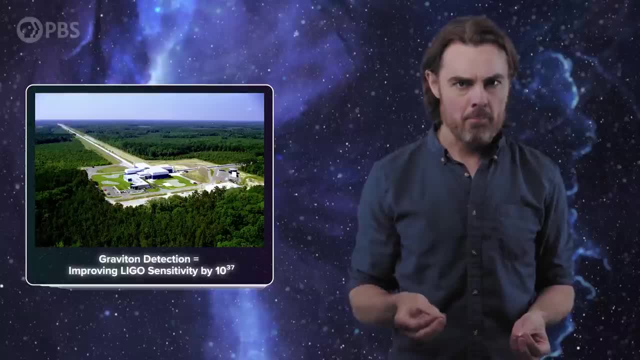 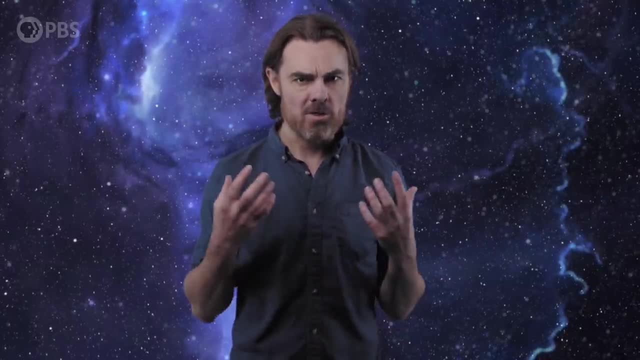 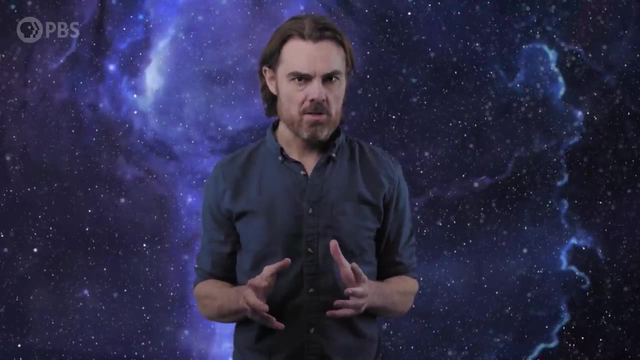 That sounds challenging, but surely not impossible To see just how science fiction-y. let's simplify our gravitational wave detector. We're going to detect incoming waves by measuring the change in the distance between two masses. We'll assume the masses are free-floating in space, but the argument also works for. 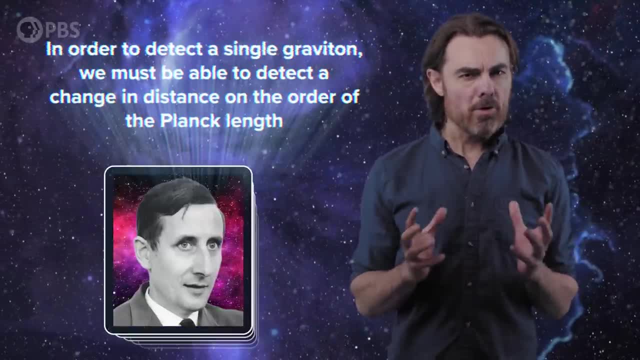 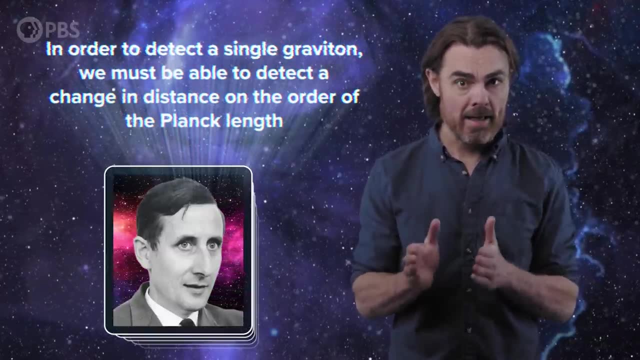 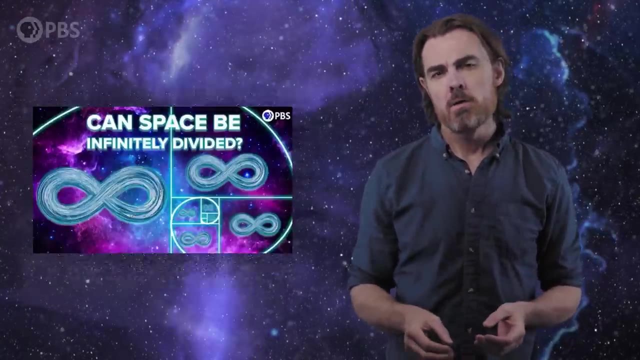 masses that are fixed to a device. Dyson argues that, in order to say that we detected a single graviton, we'd need to be able to measure a change in distance on the order of the Planck length, and that this requirement is actually independent of the frequency of the graviton. 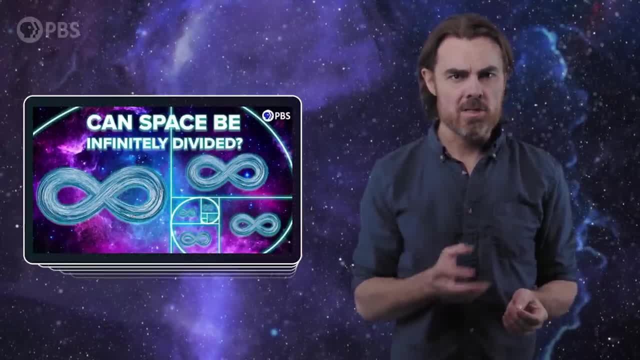 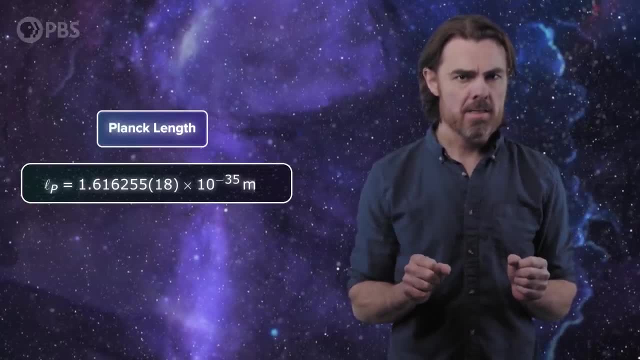 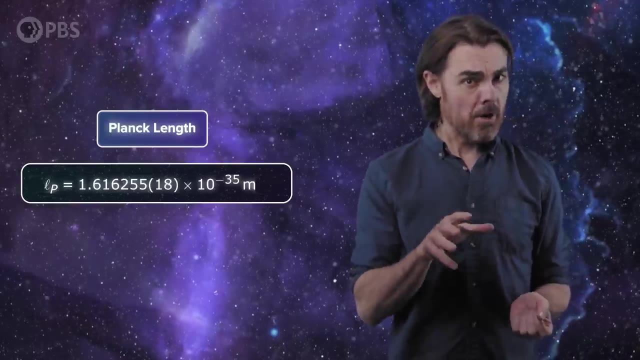 You might recall from previous videos that the Planck length is essentially the smallest distance that we can consider before the meaning of distance and space breaks down. It's a pretty small distance. So what sort of device could measure a change on that scale? For our simplified gravitational wave detector, the question becomes: what combination of masses? 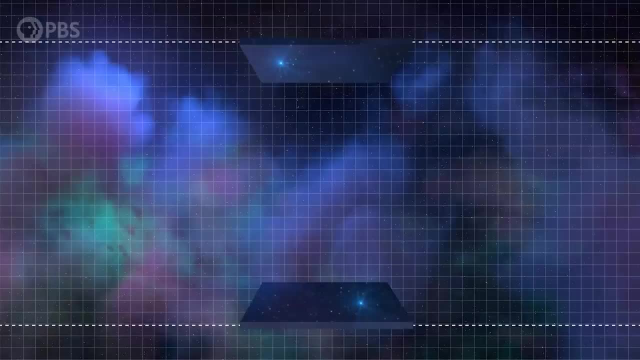 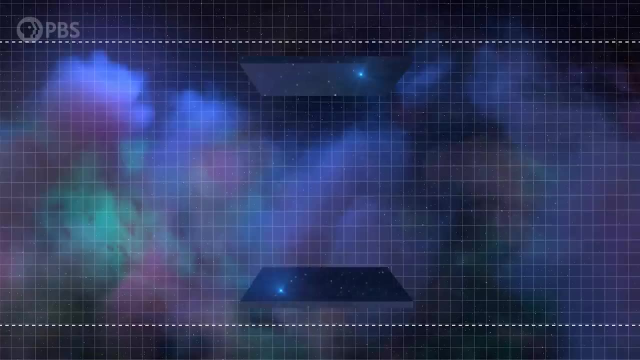 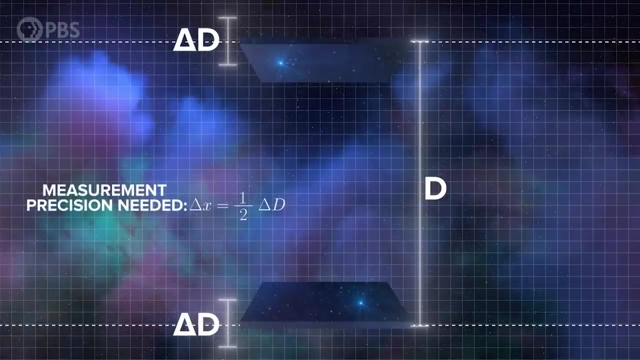 and distances between them would be. As our lonely graviton passes our detector, the masses move in and out by tiny amounts. In order to be sensitive to that tiny change in distance, we need to measure the positions of each of those masses with a precision equal to half of that change. 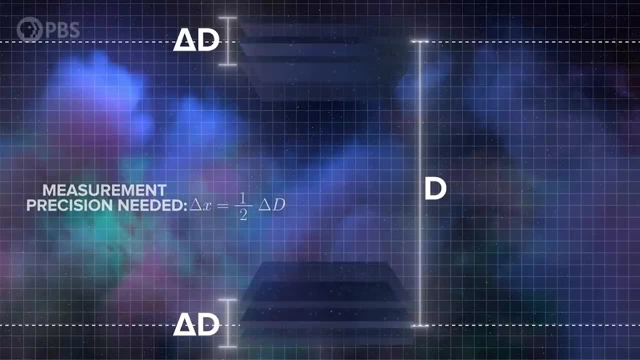 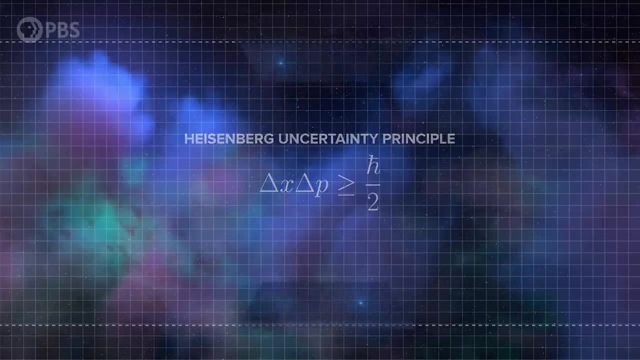 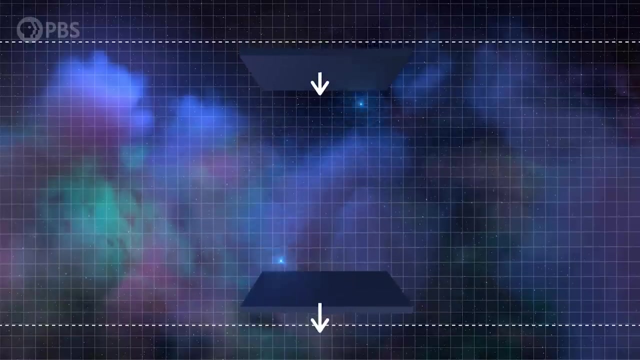 But the precision with which we can measure those mass positions is limited by the Heisenberg Uncertainty Principle, which by now you're very familiar with. While a mass is being moved by a graviton, It's speed changes. It changes roughly by the distance it travels, divided by the time it takes for a single. 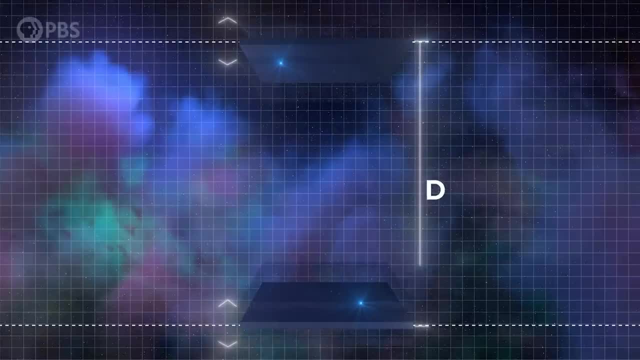 graviton to pass by That time is just the separation of the masses divided by the speed of light. That gives us the variation in the speed during our measurement. Multiply that variation by the mass itself and we get the change in momentum due to the 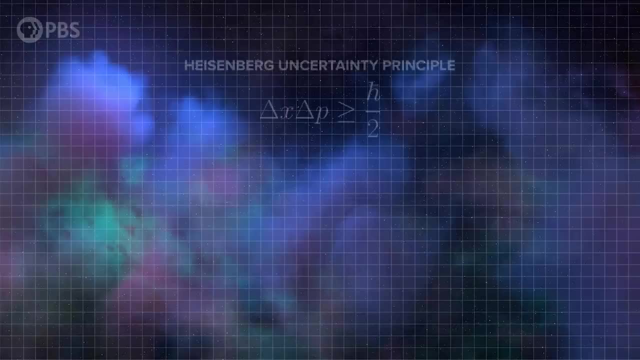 passage of the graviton. So now we have an estimate for the uncertainty in the position needed to detect the gravitational force, the graviton- and that's just around half the Planck length- As well as the uncertainty in the momentum generated by the motion of the masses caused. 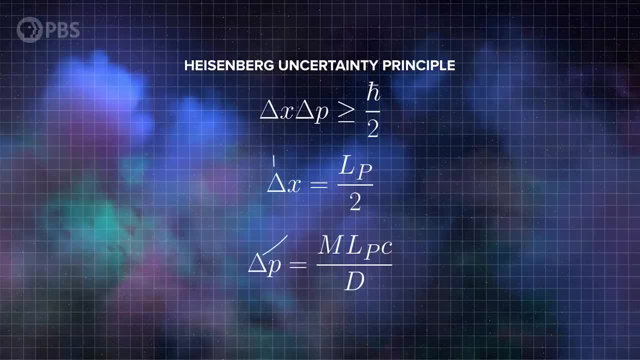 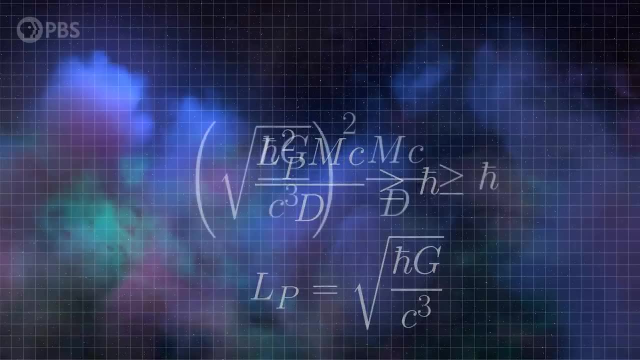 by the graviton. If we plug these into the Heisenberg Uncertainty Principle, we get a relationship between the masses and their separation. in order to be able to detect a single graviton, It's a simple enough equation: The mass separation has to be less than or equal to the gravitational constant times. 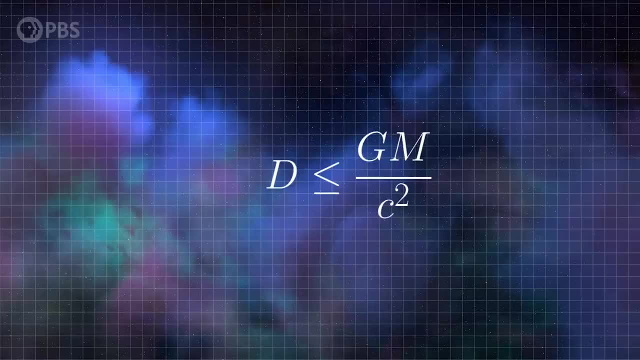 the mass of the masses divided by the speed of light squared. But that expression of the gravitational constant times- the mass of the masses divided by the gravitational constant times, the mass of the masses divided by the mass of the masses- is very familiar to all physicists and is very bad in this context. 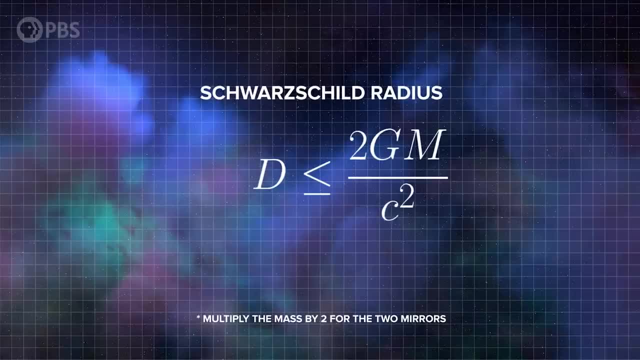 It's the expression for the Schwarzschild radius. Any mass compacted to a size smaller than this radius becomes permanently trapped by its own gravitational field. It becomes a black hole. This is really strange. We found that a gravitational wave detector capable of detecting a single graviton inevitably 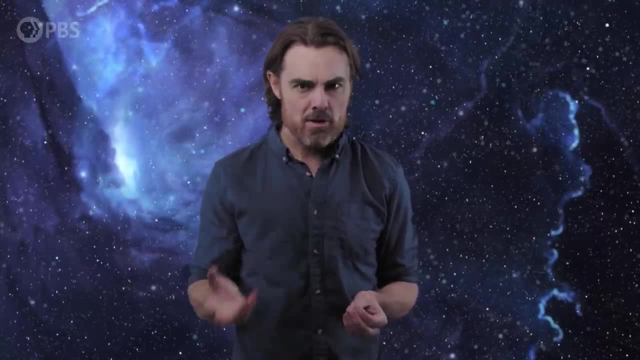 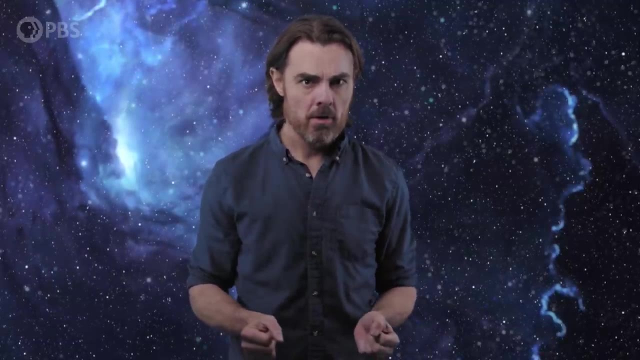 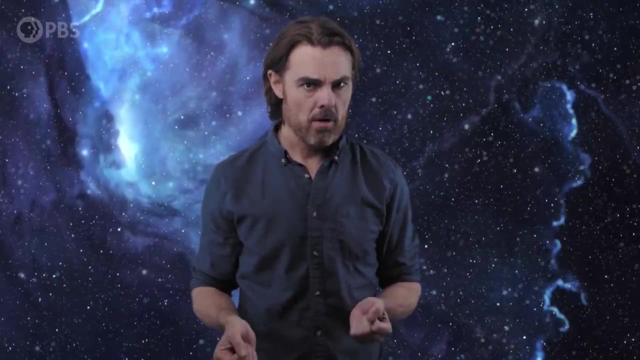 forms a black hole. That means, even if it detects the graviton, it swallows any information about that measurement and so prohibits us from confirming the graviton. Really, any attempt to measure distances smaller than the Planck length threatens black holes, as we have discussed before. 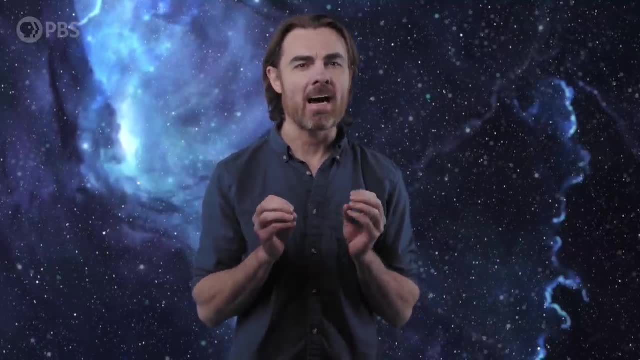 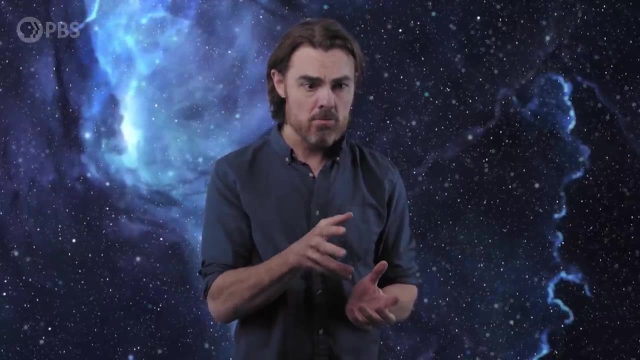 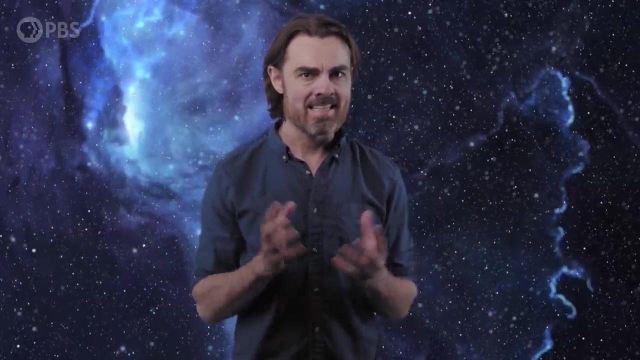 So it seems that nature isn't just conspiring to thwart our theoretical arguments for quantum gravity, but also to stop us from building the detector. we'd need to test these theories. None of this means that gravity isn't really quantum or that the existence of the graviton 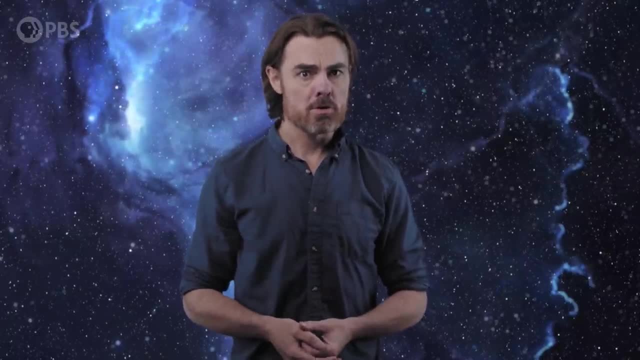 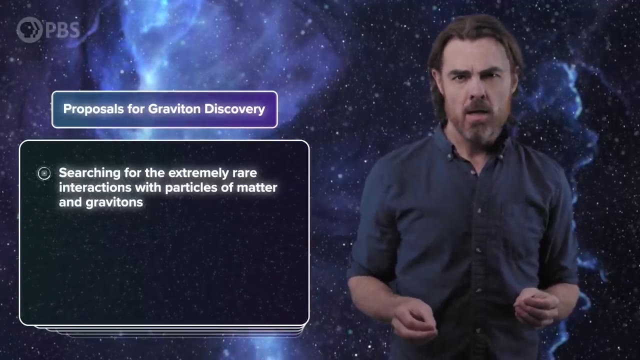 can't be ever proved. There are several proposals for how to do this, like searching for the extremely rare interactions with particles of matter and gravitons, But these events are going to be so rare that it may be practically impossible to see enough of them.